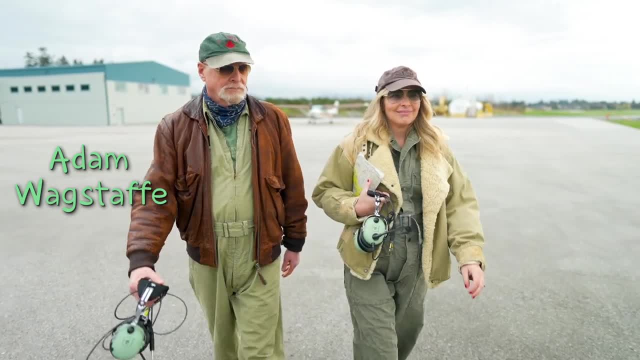 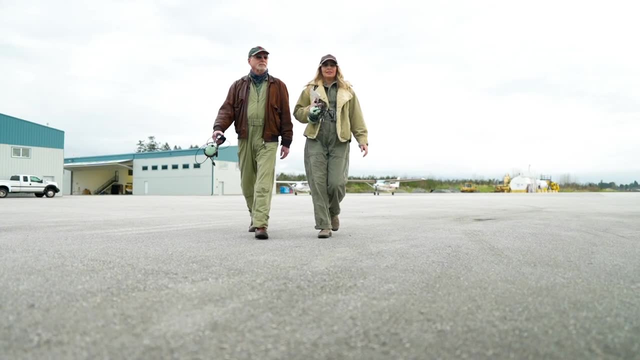 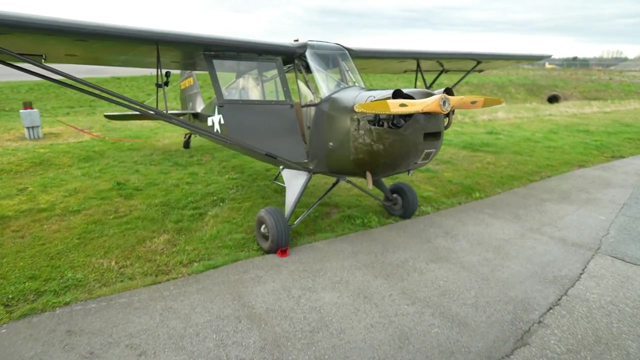 pilot and the one that got me interested in flying. When I was 12 years old, I joined the air cadets and my dad took his first flying lesson. He was inspired by his great uncle and World War II pilot. These days, my dad and I fly together in his 1943 World War II tail dragger, An Aronca L3B. 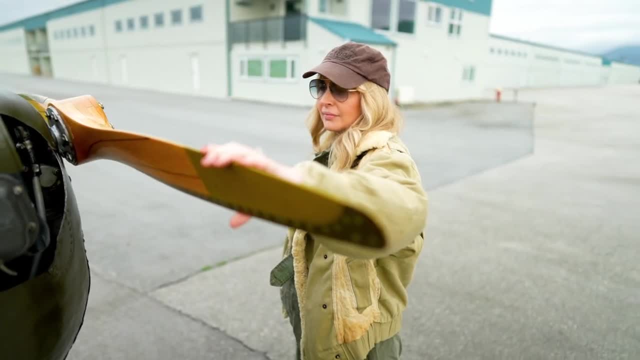 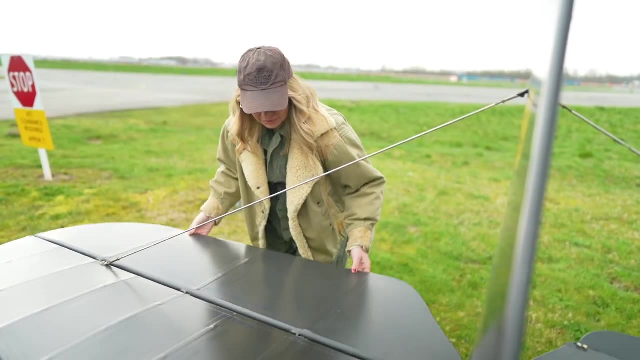 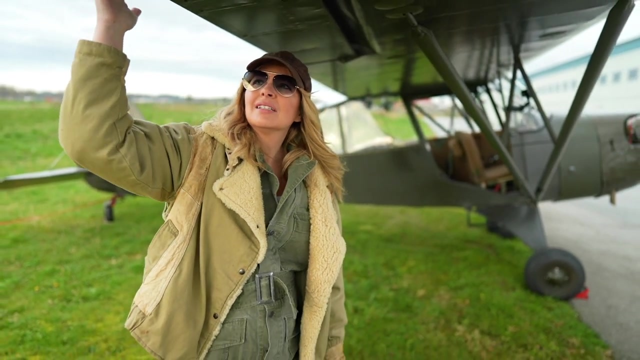 used by the US Army for observation and liaison, to be exact. And yes, I have to reconcile my carbon footprint with being a private pilot. Carbon credits do help, But it was actually getting my pilot's license as a teenager that I was first introduced to meteorology and eventually climate change. The jet stream is 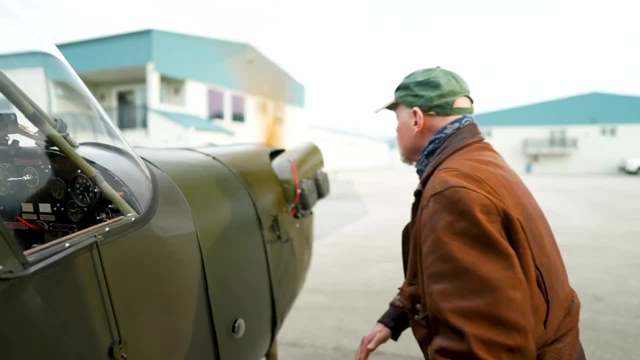 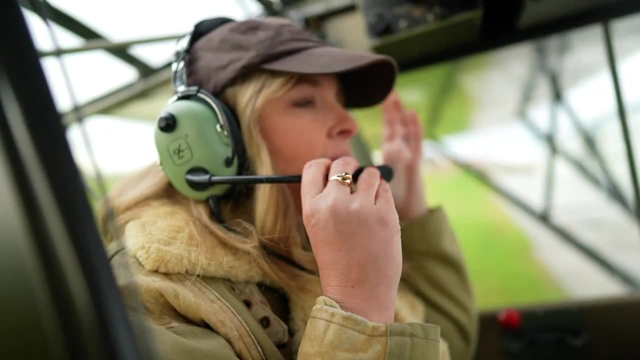 where planes catch a ride in what is essentially the highway in the sky. Okay, not this exact plane, This one does better closer to the ground, But it's that very view. This is the view of the meandering rivers down below as we navigate, the winds and the weather. 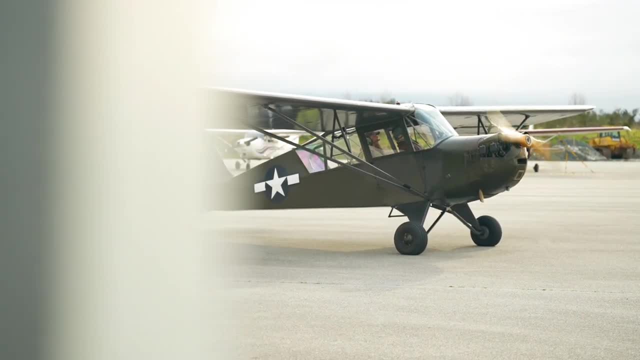 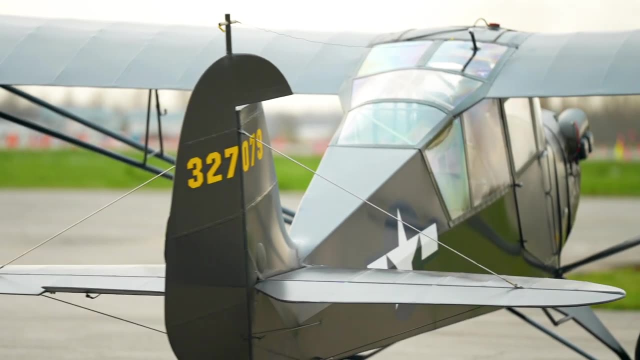 around us. that has me thinking about the similarities between what's happening above our heads and below our feet. The same conveyor belt that helps give a boost to the big planes is what carries weather systems around the world, And it's that weather that is coming. 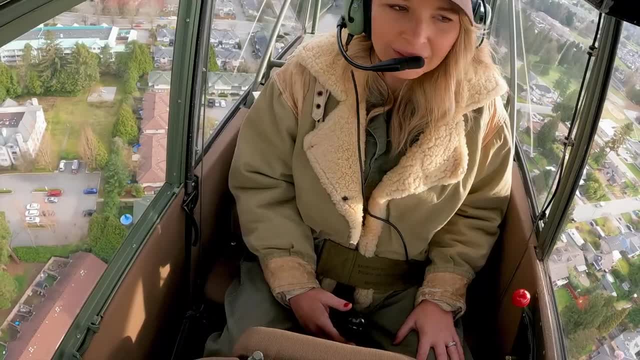 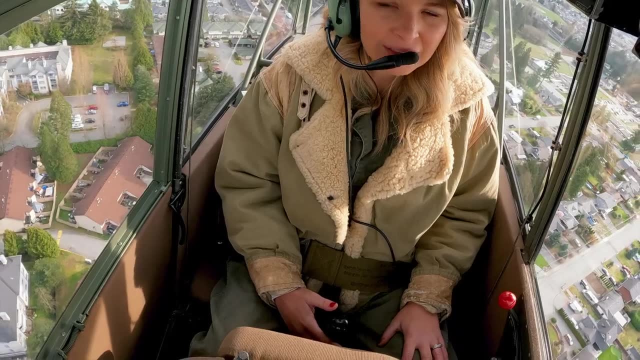 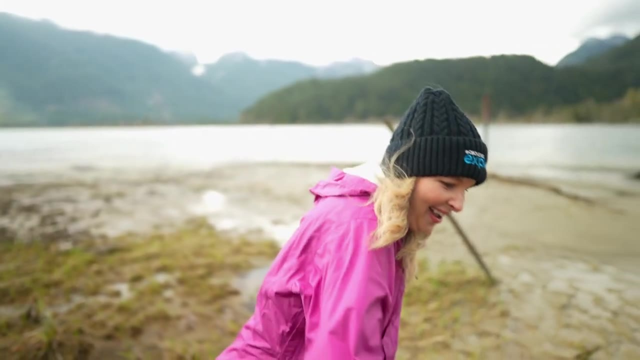 with greater frequency and intensity because of our warming climate. As a meteorologist, I want to know more about how these conveyor belts are changing And, as a pilot, well requesting permission for a flyby To learn more about these elusive rivers in the sky. 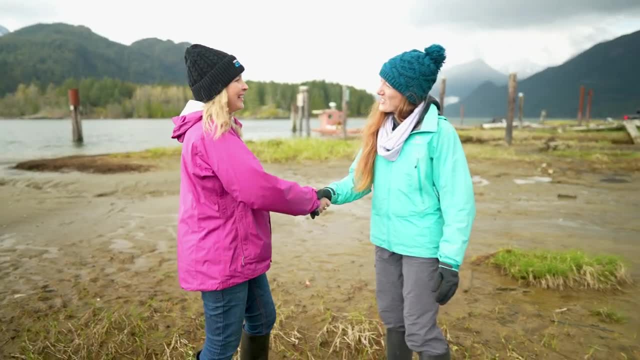 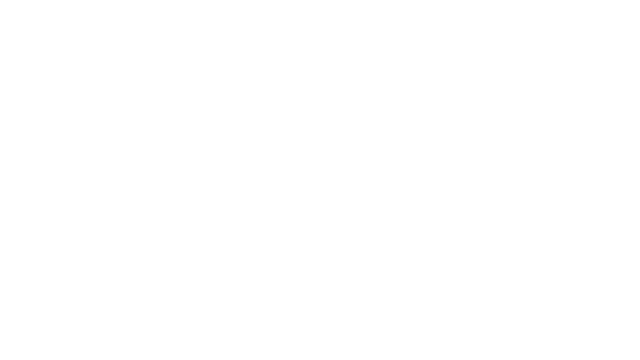 we went from a bird's eye view to a fish eye view and met up with atmospheric scientist Rachel White in the Pitt River, Literally in the river Right where the Pitt Lake empties into the river- a stunning backdrop for bird and weather watchers alike. 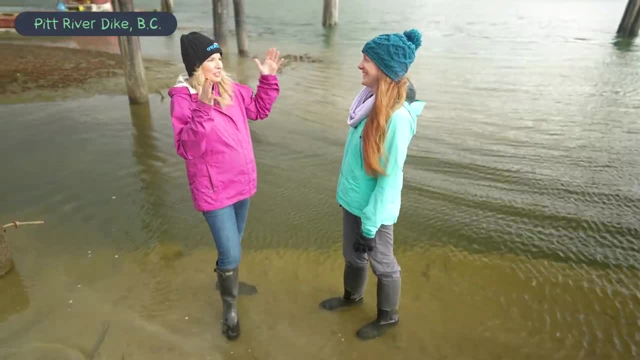 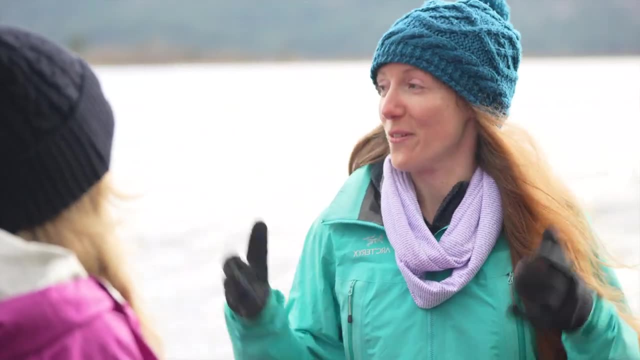 So we're standing in the Pitt River. How is it? How does the jet stream behave? like the river? That's a great analogy for what's going on with the jet stream. And so if we think about rivers, we've got this flow of water going in one direction And you know, we can think about. 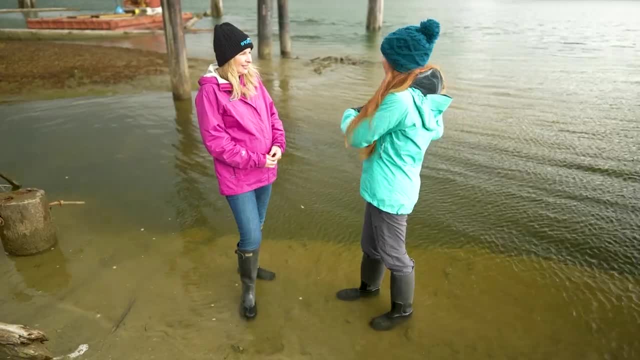 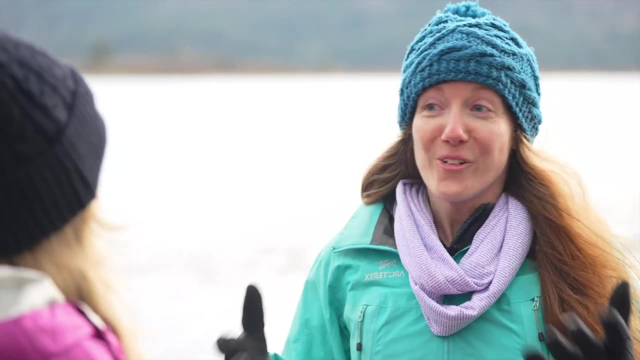 the storms that the jet stream are bringing along, like some of the eddies that we might see in the river. You see that they get advected, They get taken along by the flow of the river And also, if you think about rivers, you think they do meander. You see these loops. 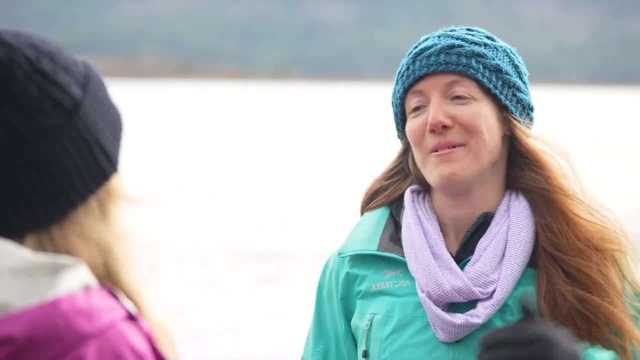 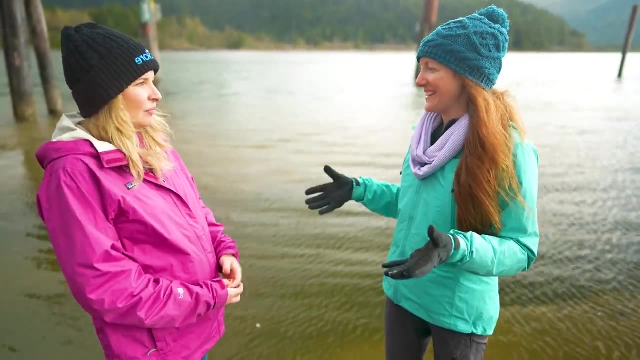 They're on a different time scale And that's what's happening in the jet stream, And so the jet stream is creating these meanders and these loops, and they're changing on a time scale of sort of days to weeks Rather than millennia. 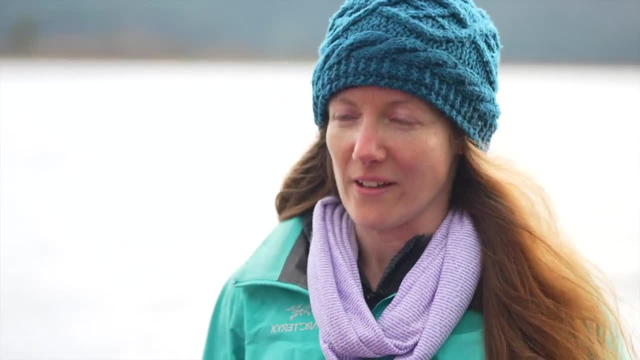 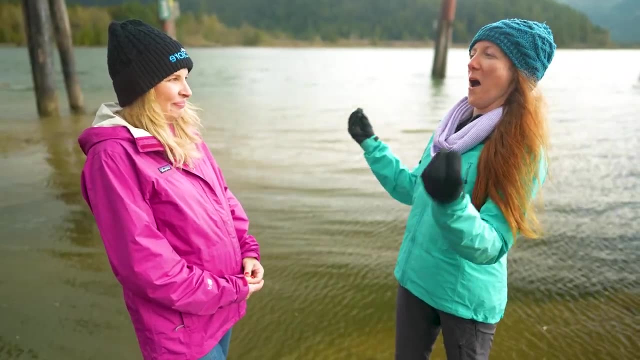 Exactly Which is what's happening with the river. But it's sort of that same thing of you know you have pieces of river joining other bits of river. When we look up in the jet stream, it's not actually at any one point, just one smooth jet. You've got all of these little. 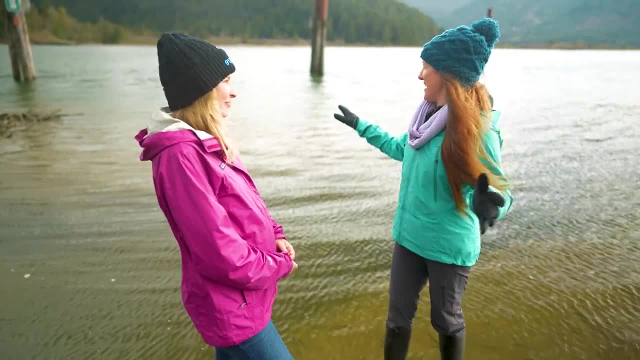 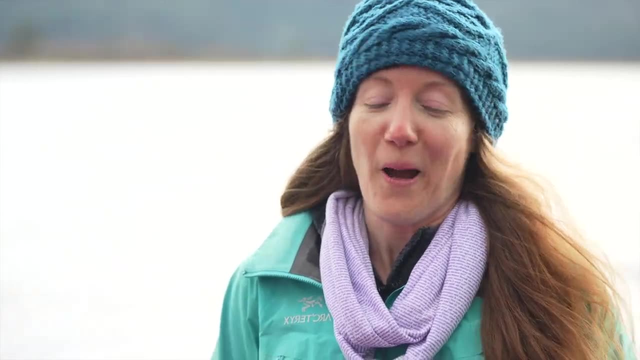 bits of the jet stream. They curve around And the jet stream is a lot wider than this river is, And so up in the atmosphere the jet stream is hundreds of kilometers wide. But you know, some of the aspects are very similar. 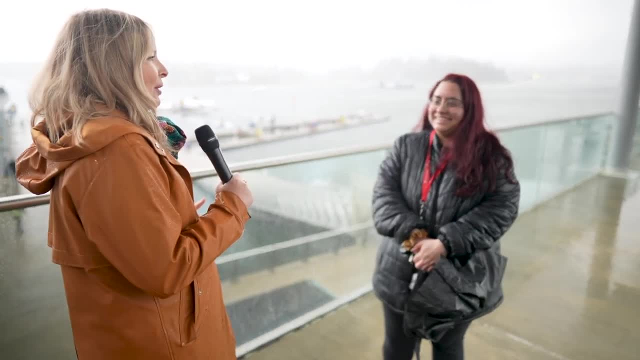 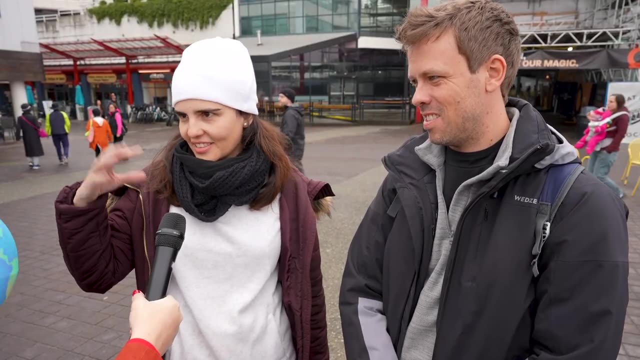 Do people know this? What can you tell me about the jet stream? The jet stream Got the wind and the sea, like the currents and stuff like that, But I don't know much- And of course, the sun if it's summertime or wintertime. that's all I know. 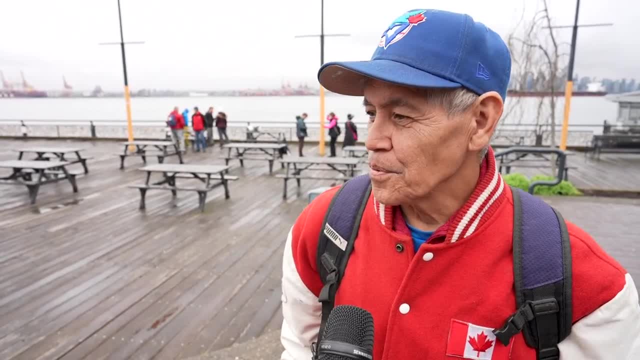 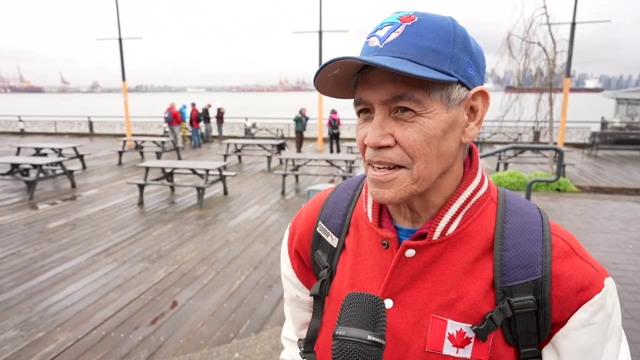 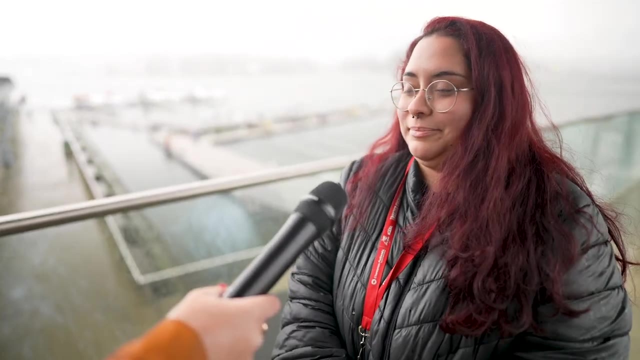 It's constantly moving And if you really look at the weather and how nature is, you can pretty much see kind of gives you a little message about what's coming up. I mean, I know like the oceans move because of like the moon, right. 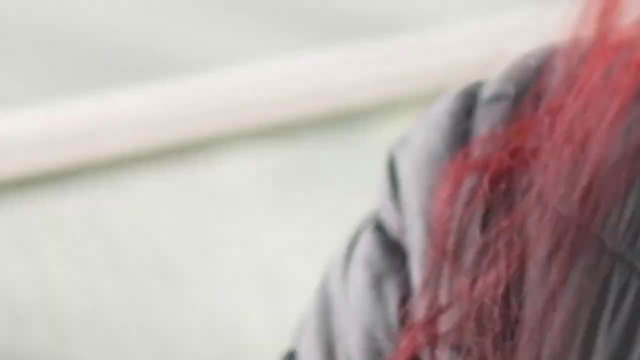 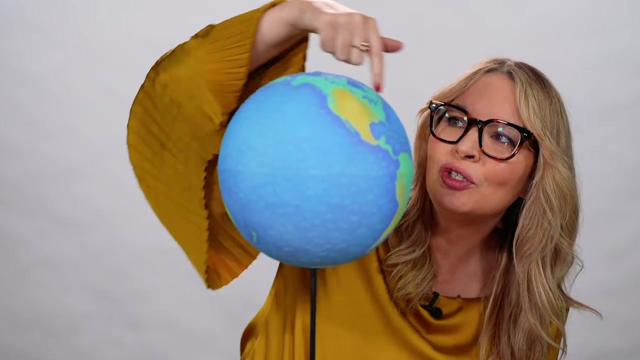 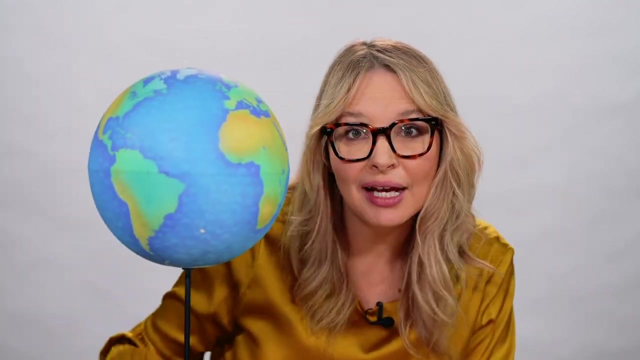 I don't know if, like, maybe it's the same thing or something close to it- The Earth has not one, not two, but four primary jet streams that circle the globe: Two around the polar regions and two around the mid-latitude regions. And that's because the Earth isn't 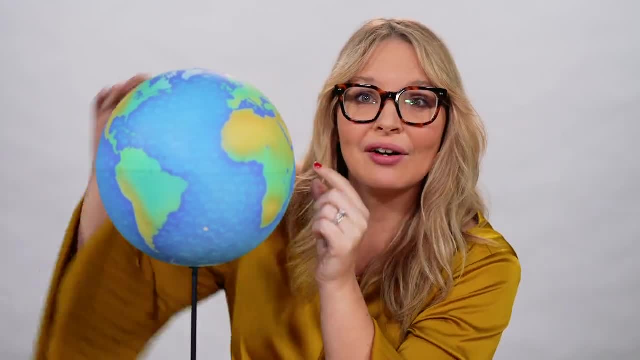 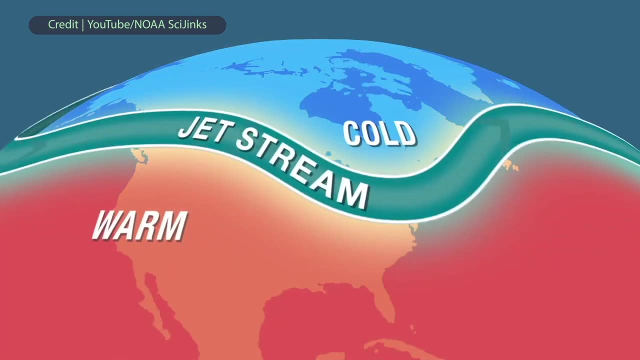 heated evenly. The sun's most direct rays hits the equator and we get the greatest temperature differences where those primary jet streams form. They can travel between 175 and 400 kilometers per hour, So that's why commercial jets often hitch a ride traveling west to east. 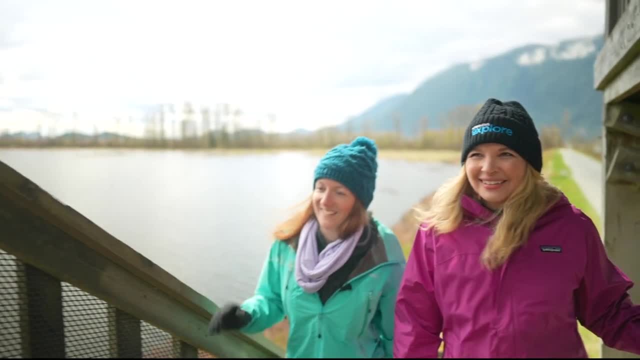 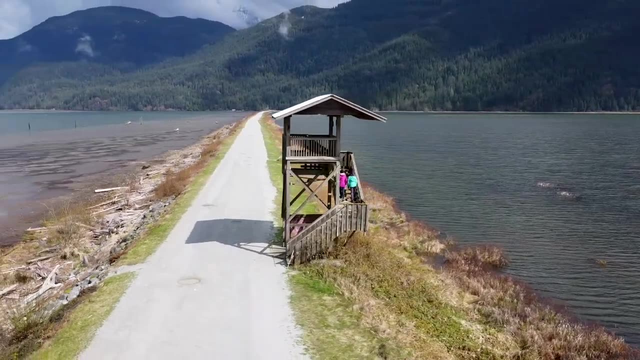 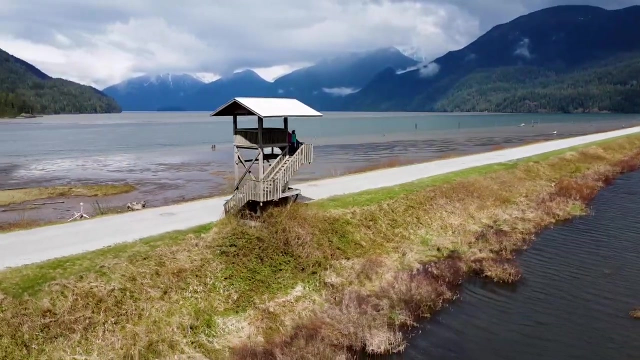 Okay, Rachel, what's going on way up there that makes weather so extreme down here? Yeah, that's a great question, And whereas when we think about weather extremes, we obviously think about what's happening at the surface, because that's what's impacting us, 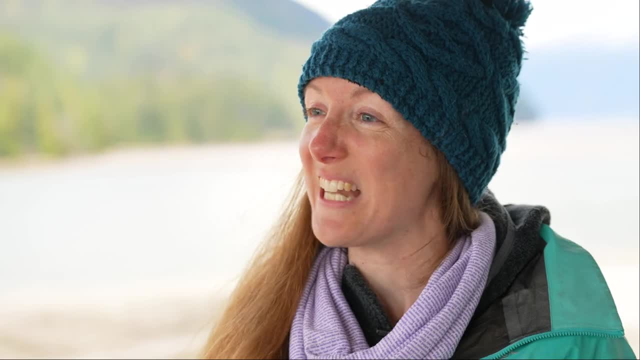 But when scientists and forecasters are sort of looking at this, they're usually actually looking at what's happening at the surface And that's what's impacting us. But when scientists and forecasters are sort of looking at this, they're usually actually looking at what's happening up in. 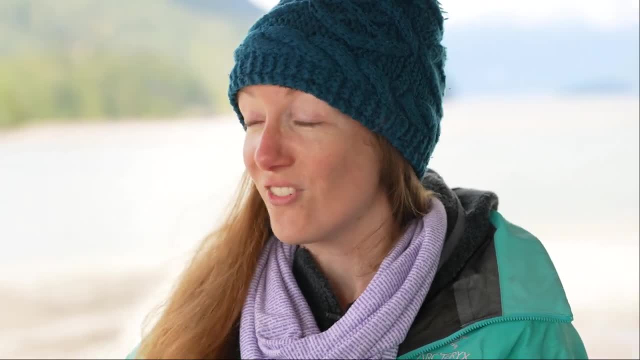 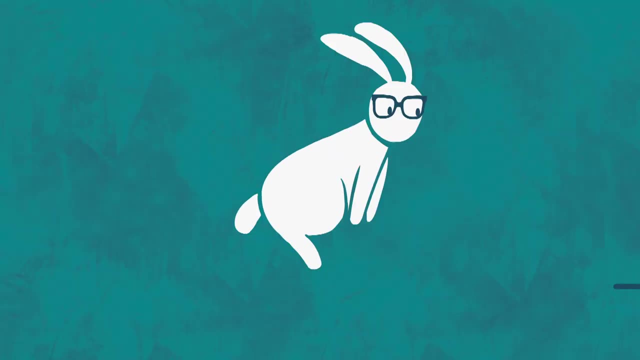 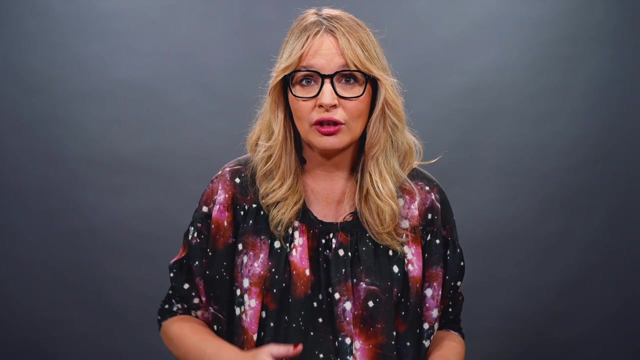 the atmosphere, And when I say up in the atmosphere, it could be as far as sort of nine kilometers above the surface. Okay, hold that thought. Experiment time. I want to demonstrate to you the two forces that affect the jet stream, the spin of the Earth and the temperature difference around our planet, and show you 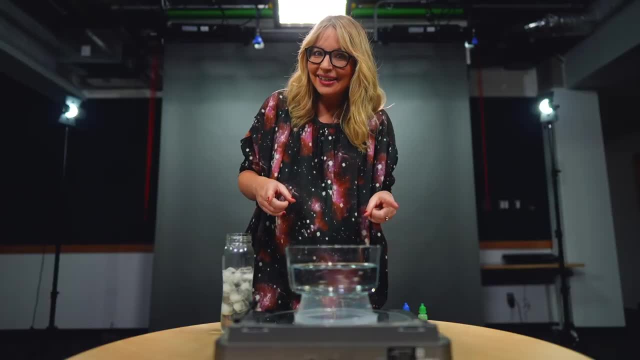 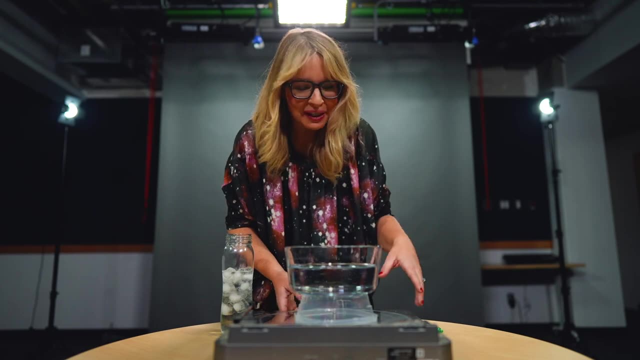 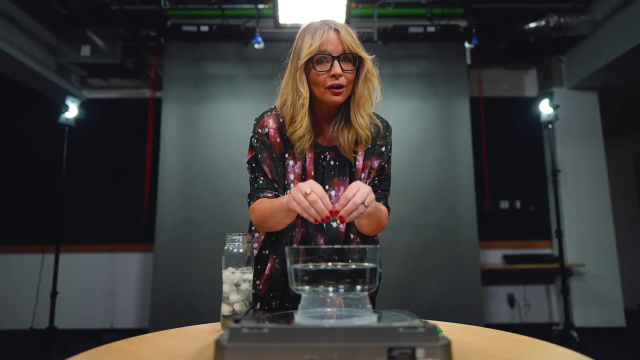 how that can drive atmospheric rivers Using household items, namely a turntable. that can drive atmospheric rivers Using household items, namely a turntable. make sure you ask your parents before you pour water on their turntable- Always wanted to say that- And various Tupperware. So this big glass bowl is a proxy for a rotating planet. The water. 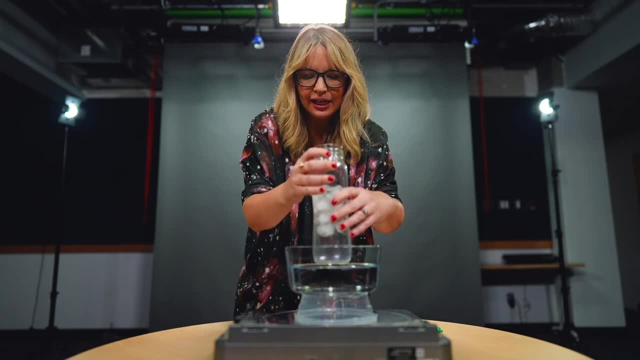 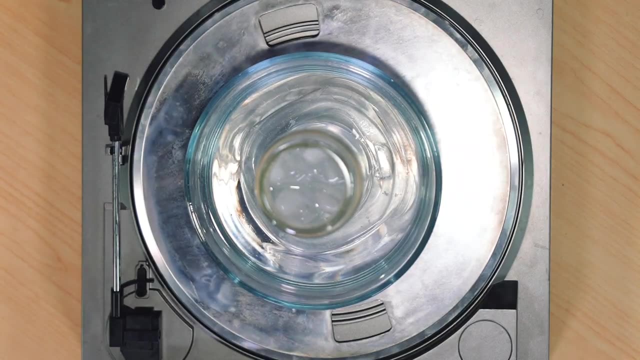 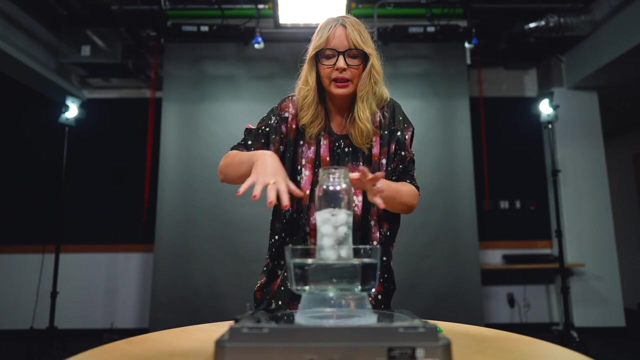 in. it is our atmosphere And this jar of ice is the pole. So you're kind of looking down on Earth from the North Pole. We're going to get this puppy spinning low RPM there And I'm going to give it a few minutes so that the water spins uniformly unperturbed. I'm trying not to pull. 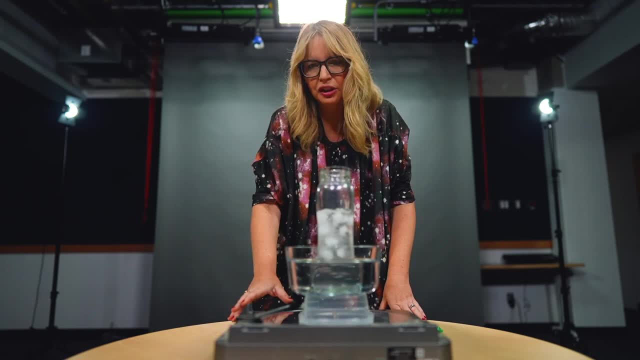 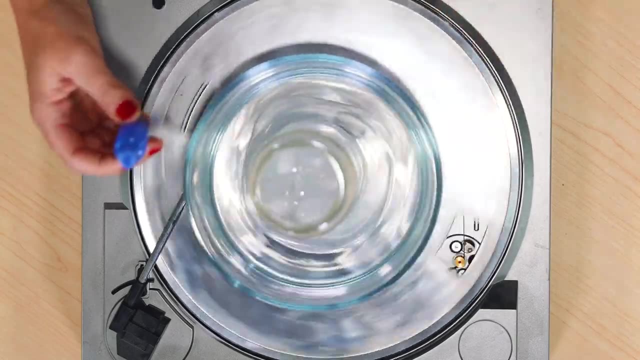 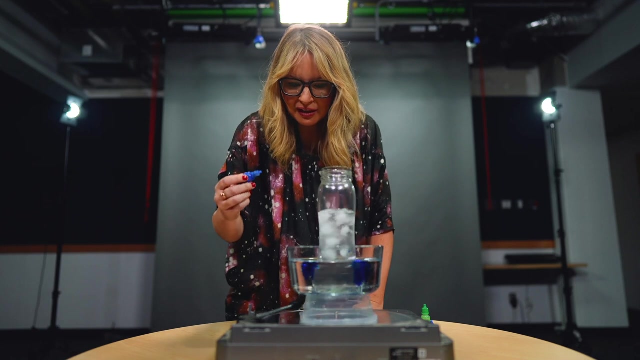 play any music while we're doing this. It'll just be scratches. Okay, first we're going to add blue food coloring close to the pole as a proxy for the polar jet stream. Let's see here just a couple of dabs Now. watch as the Earth rotates. those ribbons of cold air start to. 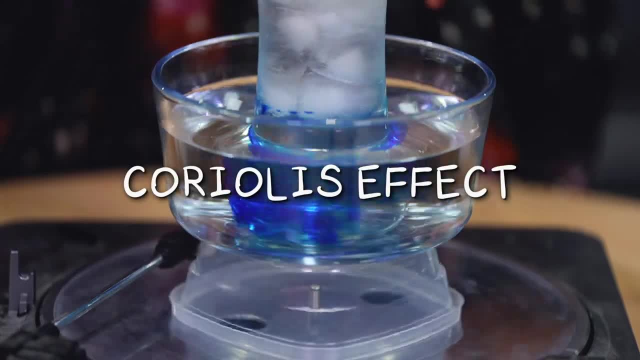 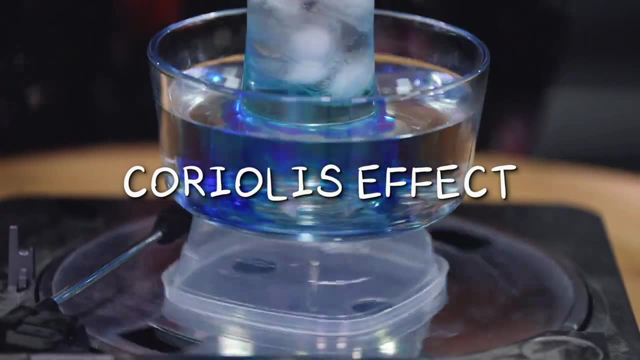 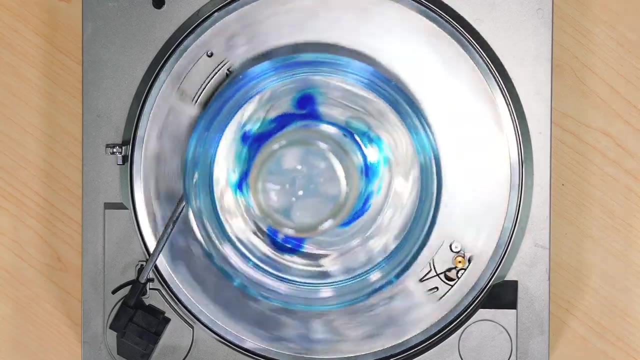 extend down towards the equator And because of the Coriolis effect, which is the deflection of air to the right because of the spin of the Earth, we start to get eddies, And those eddies are actually what our winter storms look like across Canada. Ooh, this is looking good, This. 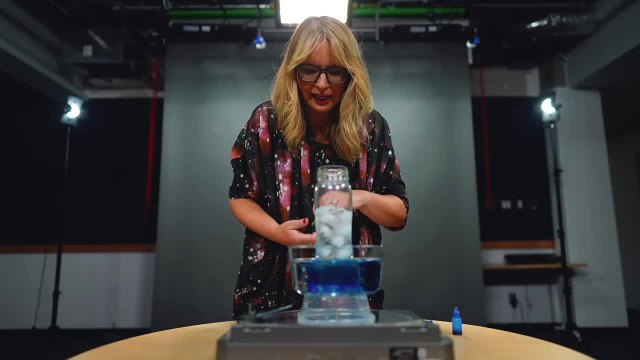 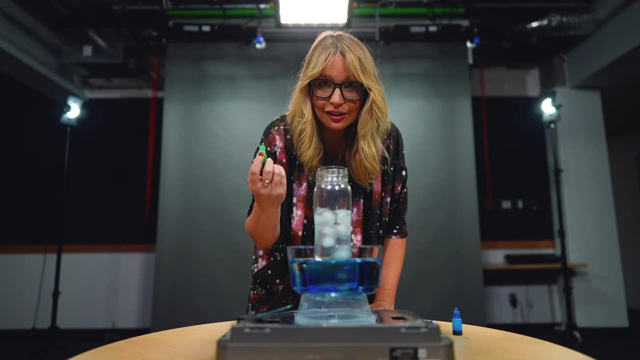 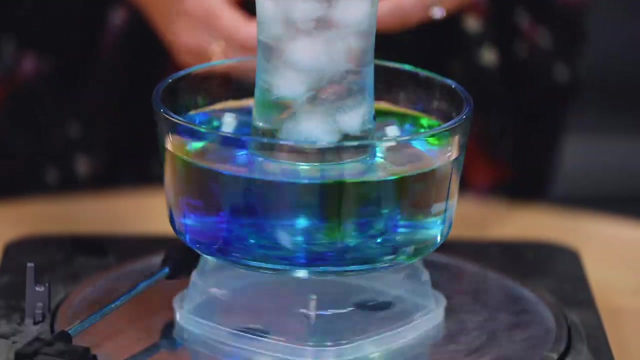 is a turbulent planet Earth right now. I love it. I count like four storms. Okay, now we're going to add green food coloring close to the equator, so the edge of the glass, And this is a proxy for a warm air. Here we go, a couple of drops here. We'll let that start to spin. 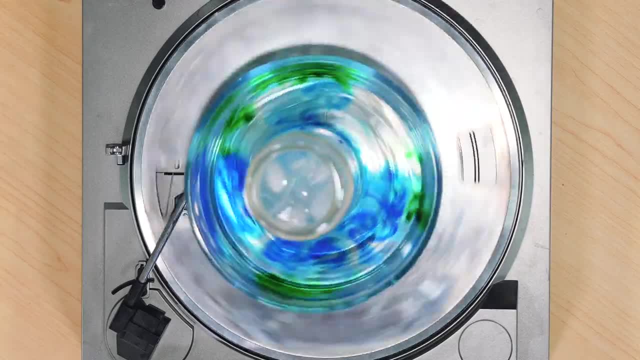 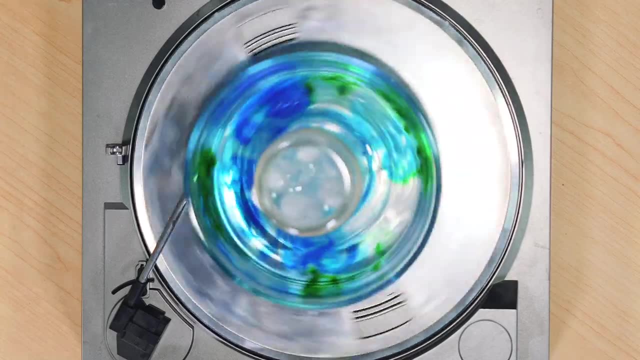 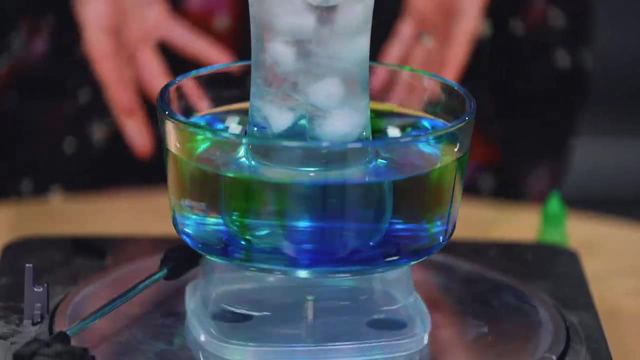 And what you'll notice is the green, warmer air starts to fill in the gaps between the cold air. You'll start to see those ribbons stretch up from the equator towards the pole, And what this is doing in reality is transporting huge amounts of warm, moist air from the equator poleward, In fact. 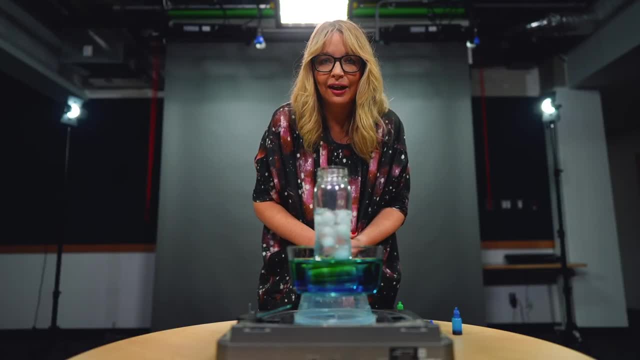 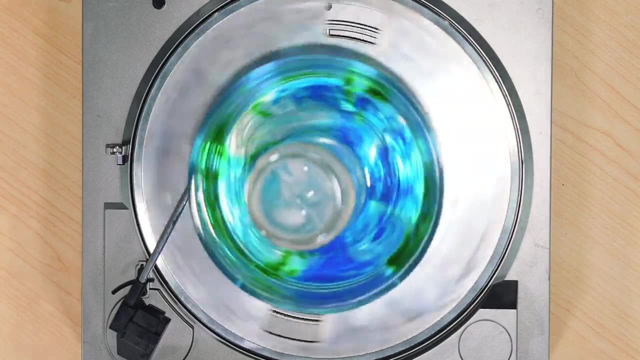 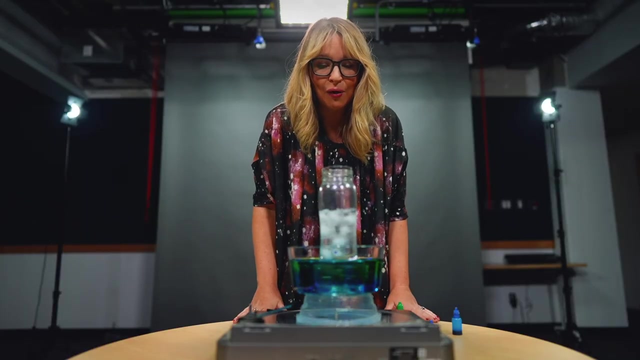 this is how the West Coast of the US and Canada gets most of its water vapor: via these huge atmospheric rivers, And that's really what you're looking at. These ribbons are atmospheric rivers that stretch hundreds of kilometers. Now, this is a very stormy planet Earth right now. 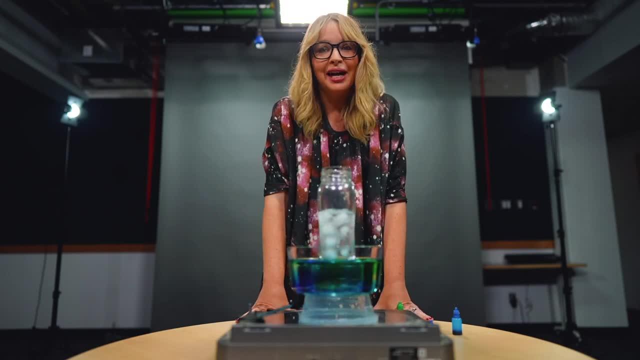 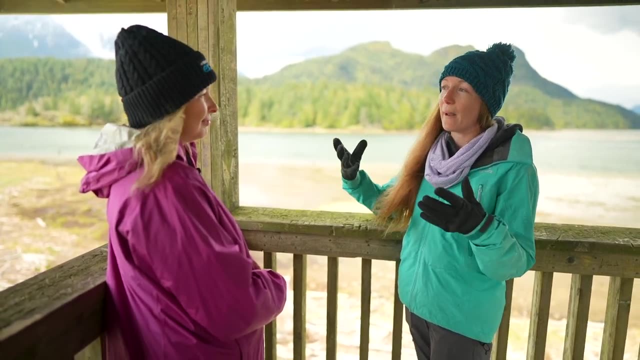 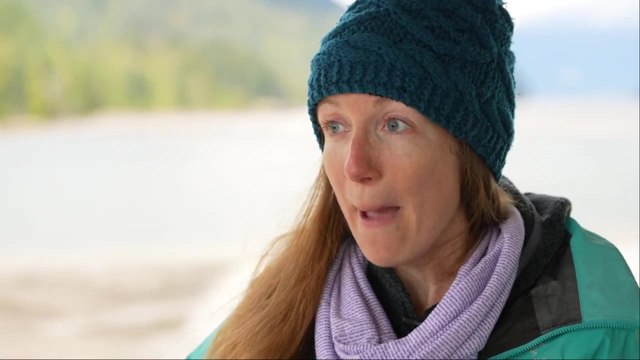 but this is actually an excellent proxy for what's happening right above our heads, And so what's happening up there is really sort of creating the systems. that's where systems are growing and developing that are going to affect the weather down at the surface, And there's different ways that extremes can happen, and all of them are affected by. 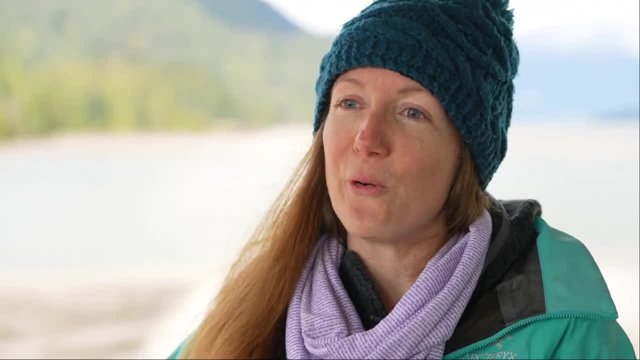 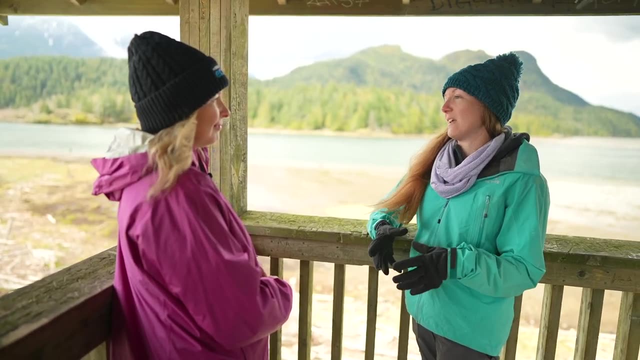 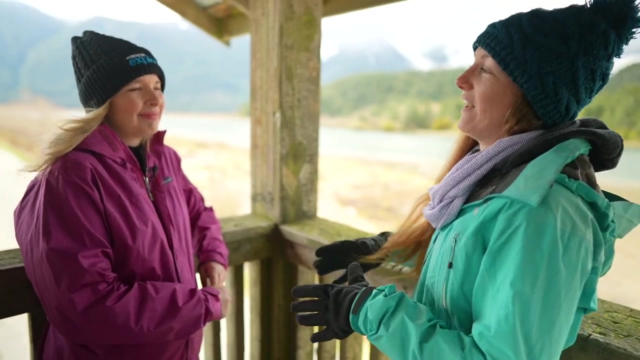 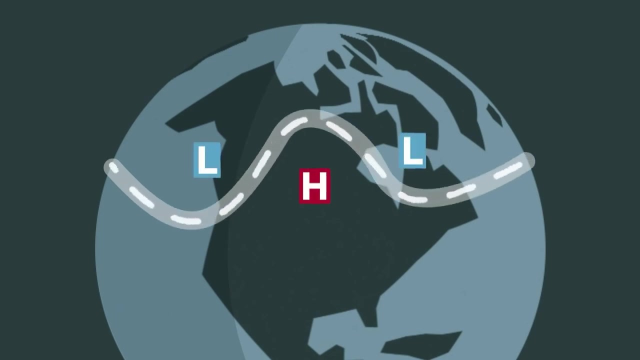 the atmosphere, And so what's happening is that we have a high pressure system that's sitting sort of over a particular region and it's staying still, And so we call this a blocking high, and it's called blocking because it sort of blocks any other weather systems that might be coming in. 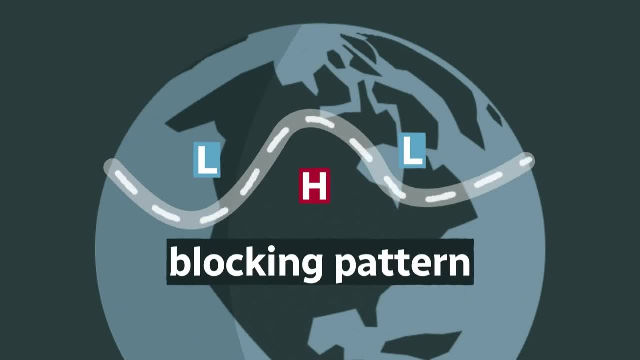 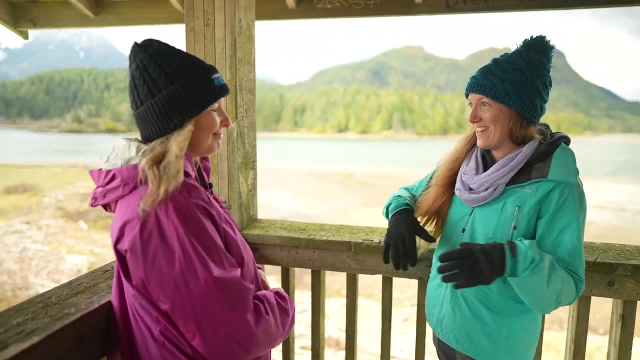 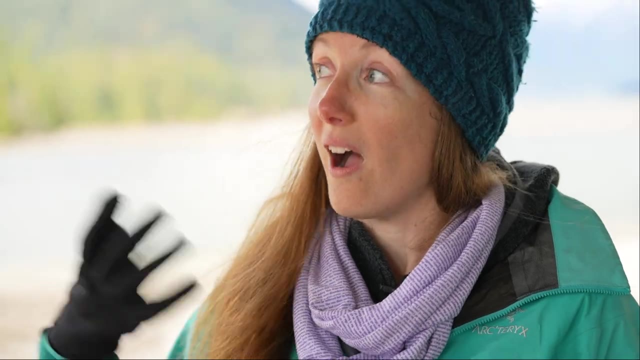 and they get diverted around this high pressure system, And then this high pressure just stays over us, And so for cold extremes. actually, it's often a lot more to do with the meanders in the jet stream up above us that end up bringing in a lot of cold air from the north. essentially, 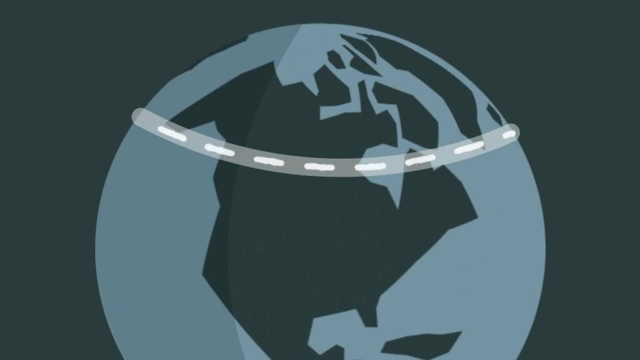 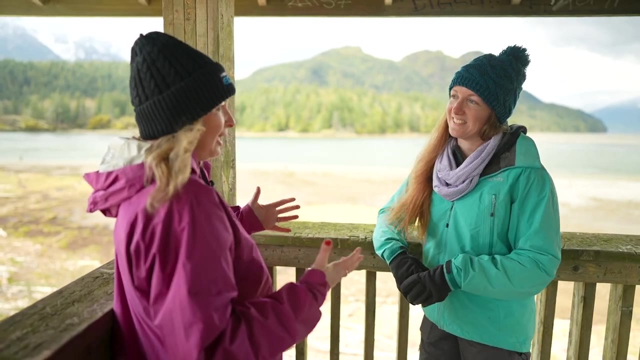 And so when we have a meander or we have winds coming from the north towards us in the northern hemisphere, this is going to create pretty cold weather here. As a meteorologist, I often think of the jet stream as the conveyor belt for weather And we look for blocking patterns.